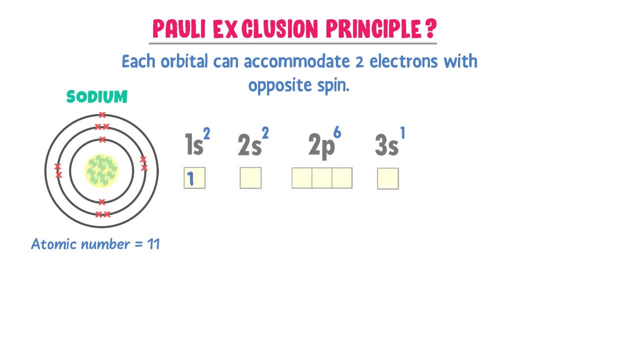 principle, the orbital of 1s and 2s can accommodate two 2 electrons with opposite spin. There are six electrons in the 2p subshell. According to Hearn's rule, firstly only one electron is placed in each orbital, having same spin, and then they are doubly filled with electrons. 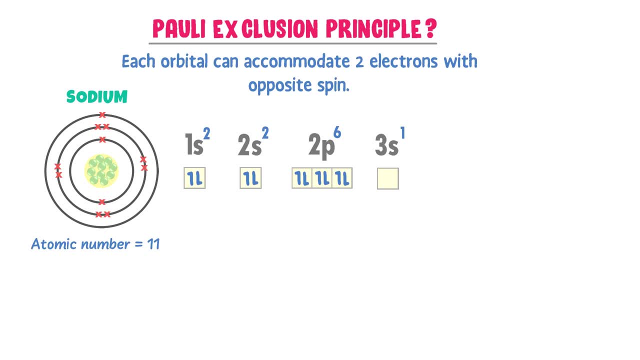 having opposite spin And the last electron is placed in the orbital of 3s. Here let me quickly revise the spin quantum number. Spin quantum number is denoted by ms. Remember that if an electron moves in upward direction, its spin quantum number, ms, is always equal to positive. 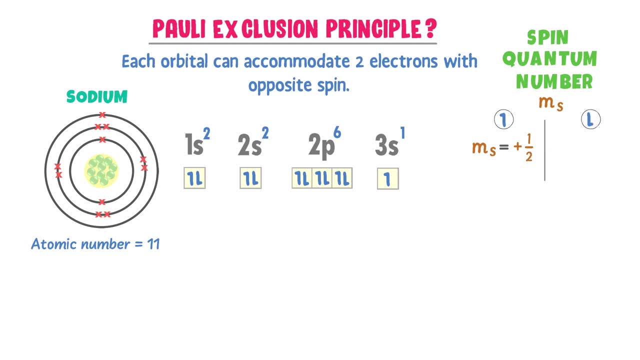 one half. If an electron moves in downward direction, its spin quantum number, ms, is always equal to negative one half. Now let me take 1s orbital. We know that there are two electrons present in it with opposite spin. I mean, one electron is present in upward direction and another electron is present. 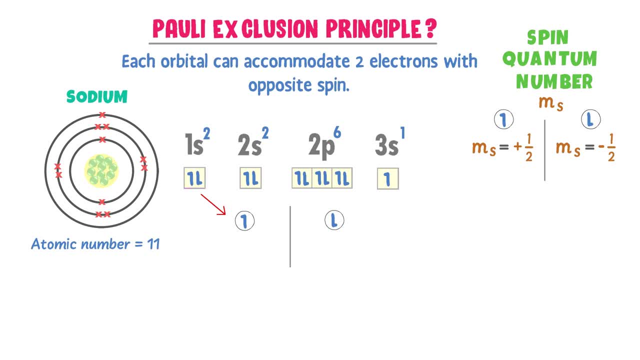 in downward direction. So the spin quantum number, ms, of this electron is equal to positive one half, And the spin quantum number of this electron is equal to negative one half. Now listen carefully. These two electrons belong to the same orbital. I mean 1s orbital. 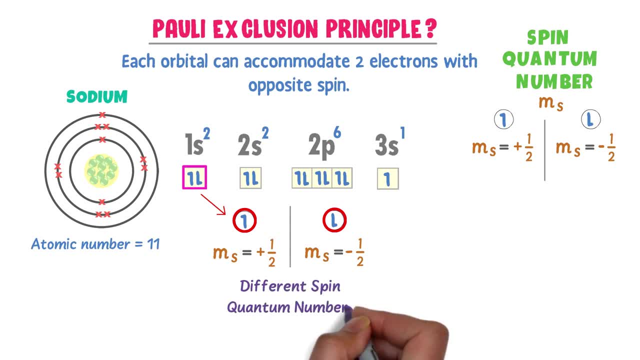 But these two electrons have different spin quantum numbers within the same orbital. Thus, to conclude this, we say that no two electrons in an atom have the same set of four quantum numbers. Let me repeat it: No two electrons in an atom have the same set. 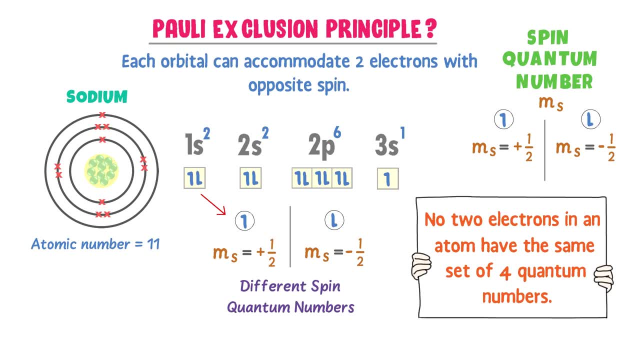 of four quantum numbers. Therefore, remember that Pauli-Baba states two important principles. Firstly, it states that each orbital can accommodate only two electrons with opposite spin. Secondly, it states that no two electrons have the same spin quantum numbers. There are two más, and. 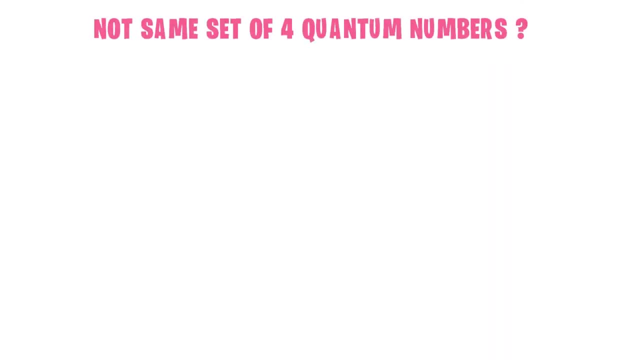 same set of four quantum numbers. Now let me teach you that. why no two electrons have the same set of four quantum numbers? Well, consider oxygen, and its atomic number is 8.. In the case of 8 electrons of oxygen, 1s can accommodate two electrons, 2s can accommodate two electrons and 2p can accommodate. 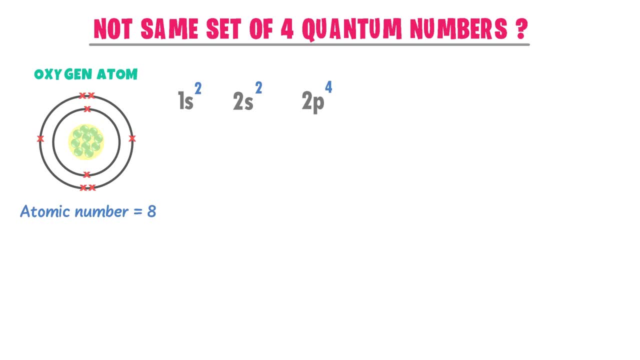 four electrons of oxygen. We know that 1s and 2s have one orbital. 2p has three orbitals as 2px, 2py and 2pz. Two electrons and 1s orbital with opposite spin. two electrons and. 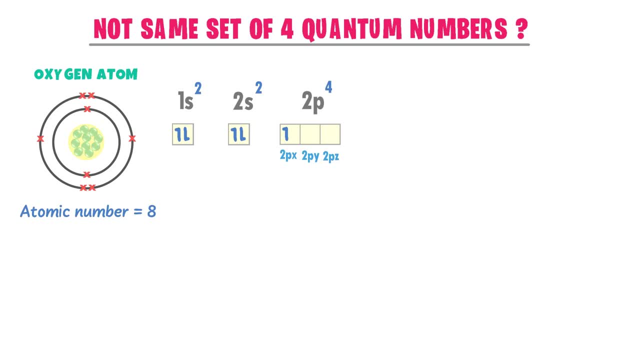 2s orbital with opposite spin. one electron and 2px, one electron and 2py and one electron and 2pz. One electron is left behind. you can place it in either orbital, but I place it in 2px. 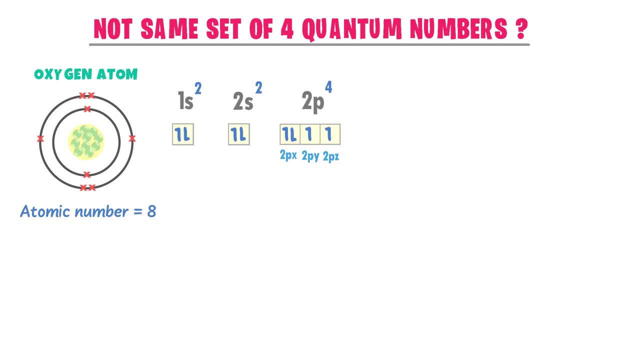 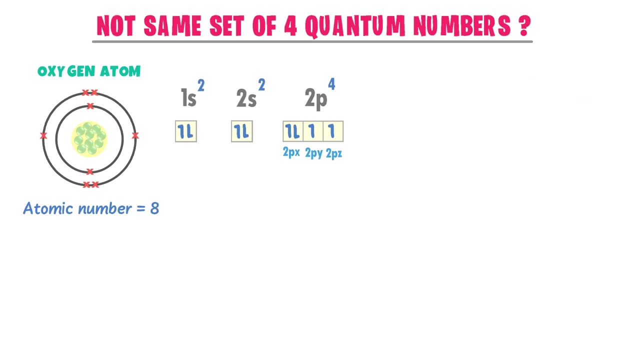 This is the electronic configuration of oxygen and its orbitals. Remember that according to Hearn's rule, you can even start filling 2p orbitals in downward direction, but all singly filled orbitals must have the same downward direction. Now let me take 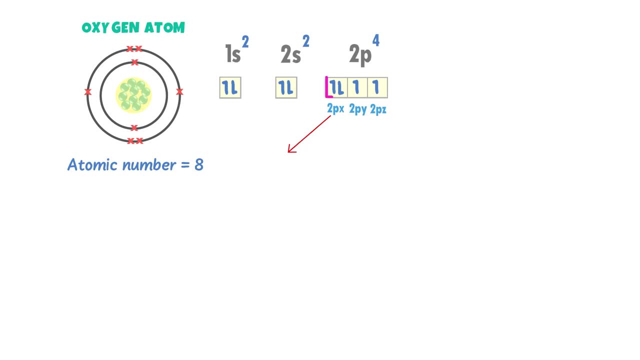 the two electrons of 2px. We know that in this orbital there is one electron in upward direction and one electron in downward direction. I am going to find the four quantum numbers of this upward electron. If you do not know how to find four quantum numbers easily, watch our lecture. 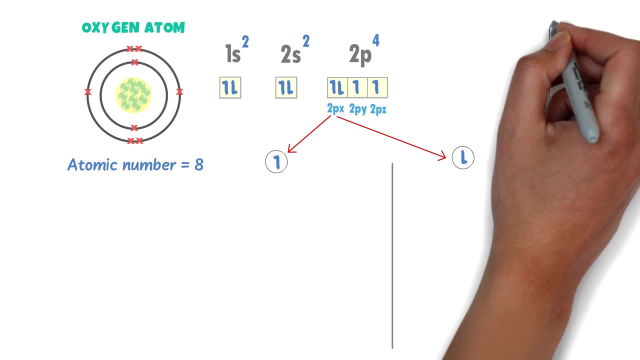 and its link is given in the description. Now always write spdf and 0123 at one side of the page. Here n is equal to 2.. For p, l is equal to 1.. When l is equal to 1, go. 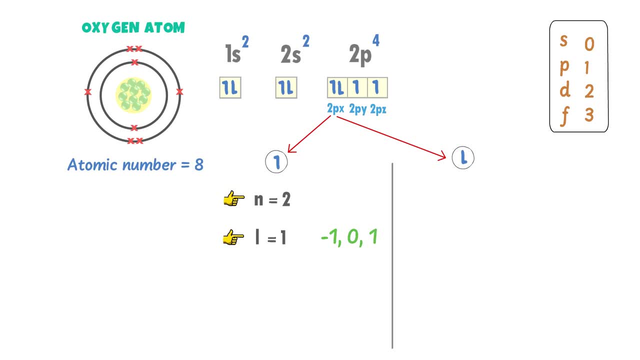 from positive 1 to negative 1, negative 1, 0, 1.. So there are three orbitals in this orbital. Now let me take the two electrons of 2px. Here n is equal to 2.. For p l is equal to 1.. When 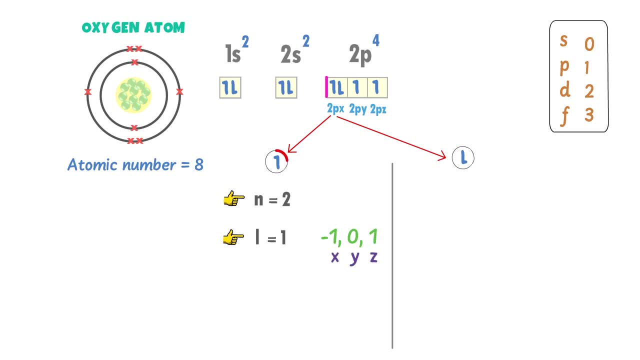 l is equal to 1, go from positive 1 to negative 1, negative 1,, 0, 1.. So there are three orbitals. There are three orbitals of l, x, y, z. This electron is in the x-orbital, so its magnetic. 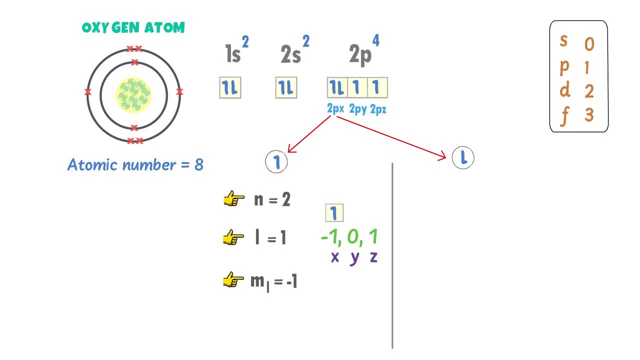 quantum number is equal to negative 1.. The direction of this electron is upward, so its spin quantum number, ms, is equal to positive 1⁄2.. In case of this electron, n is equal to 2.. For p l is equal to 1.. Go from negative 1 to positive 1, negative 1, 0, 1.. So there. 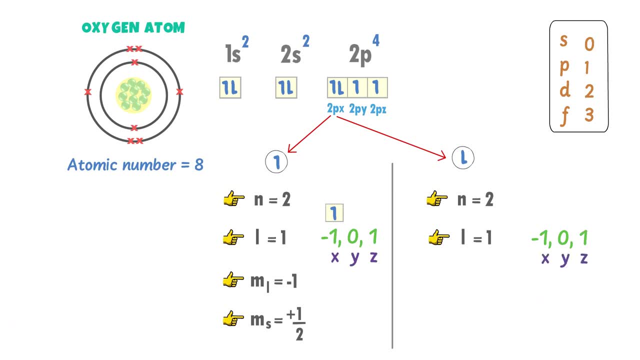 are three orbitals. in this orbital of L XYZ, This electron is in the X orbital, so ML is equal to negative 1. The direction of this electron is downward, so its MS is equal to negative one half. Now check the similarity between four quantum numbers of these two electrons. Let this is set P and. 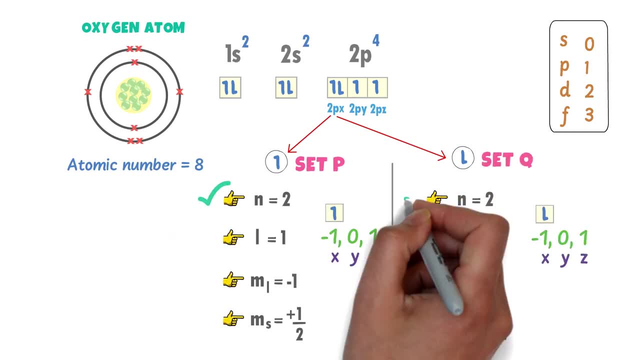 this is set: Q, N is equal to 2, N is equal to 2, L is equal to 1, L is equal to 1, ML is equal to negative 1, ML is equal to negative 1, but MS is equal to positive one half and. 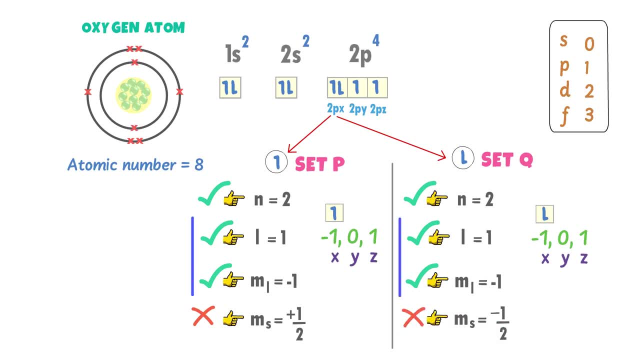 MS is equal to negative one half. These three quantum numbers for both the electrons are the same, but the fourth quantum number, I mean spin quantum number, is not the same. Therefore we say that the two electrons and two PX have not the same set of four quantum numbers. 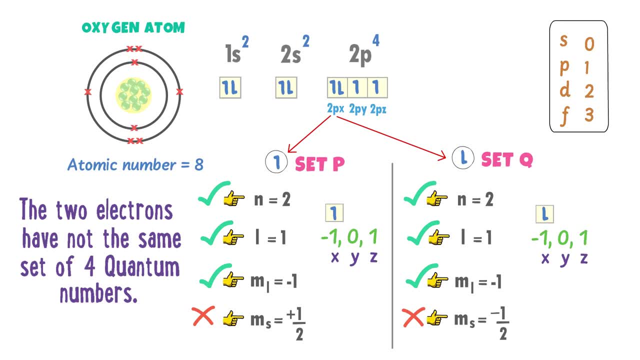 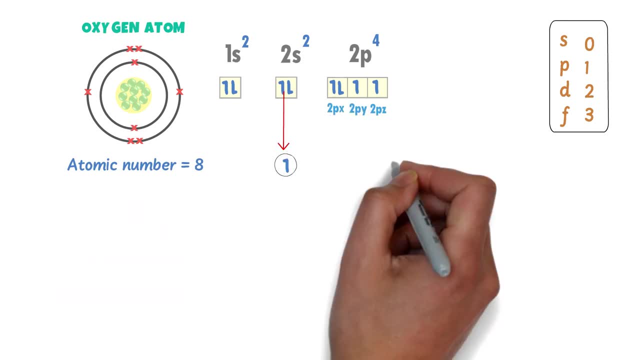 Hence it is the proof of Pauli exclusion principle. Lastly, let me quickly give you one another example. Let me take the upward electron of 2S and let me take the upward electron of 2PY. I am interested to find the four quantum. 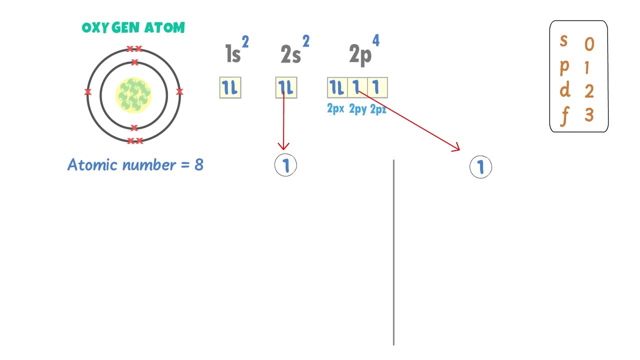 numbers of these two electrons and different orbitals. In case of 2S, N is equal to 2.. For S, L is equal to zero. Go from positive zero to negative zero, As we know that there is no positive zero and no negative zero. So this is the proof of Pauli exclusion principle. 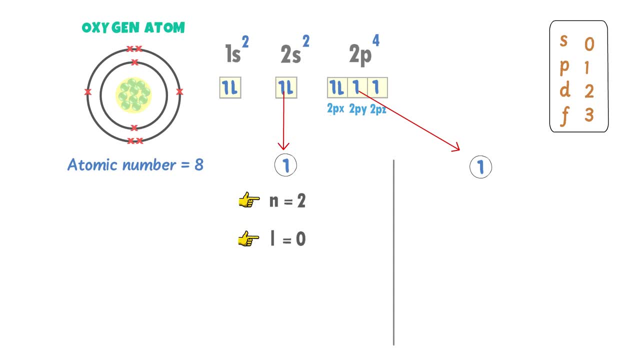 Lastly, let me quickly give you one another example. Let me take the upward electron of negative zero- Hence L has one orbital zero- and place the electron in it, So ML is equal to zero. This electron is in the upward direction, So MS is equal to positive one half In case. 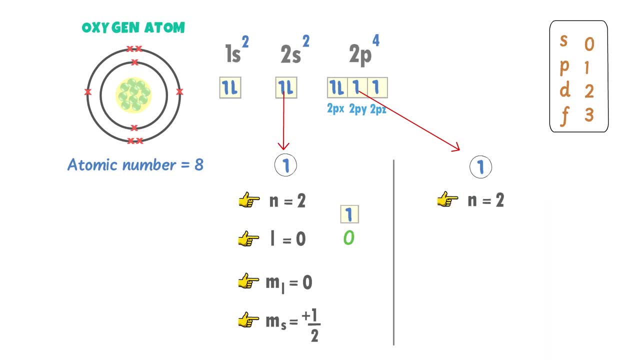 of 2PY, N is equal to two. For P, L is equal to one. Go from positive one to negative one, Negative one, zero one, So L has three orbitals, XYZ, And this electron is present in Y orbital, So ML is equal to zero. We know that this. 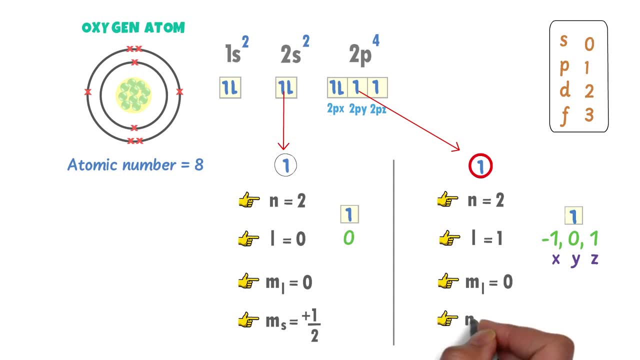 electron is present in upward direction. So MS is equal to positive one half. Let I call this as set P and I call this as set Q. Now check the similarities between these two sets: N is equal to two, N is equal to two, But L is equal to zero and L is equal to one ML. 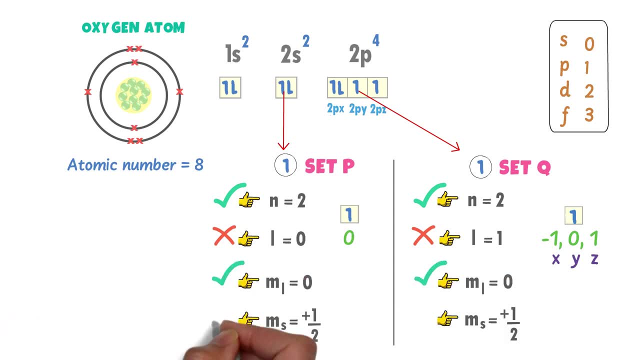 is equal to zero, ML is equal to zero, MS is equal to positive one half and MS is equal to positive one half. Here these two electrons have different values of azimuthal quantum number L. Therefore we say that these electrons, N2S and 2PY, have not the same set of four. 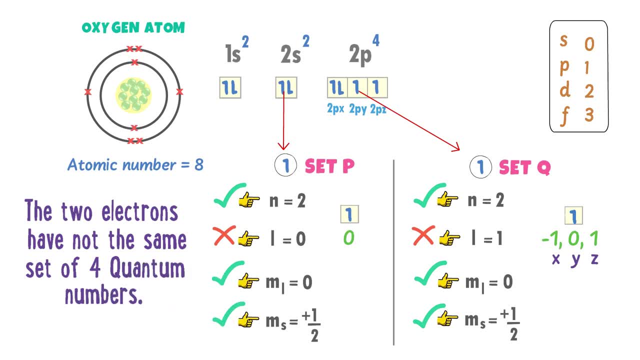 quantum numbers. It is the another proof of Pauli exclusion principle. I hope that you have learnt all about Pauli exclusion principle. Thank you very much. 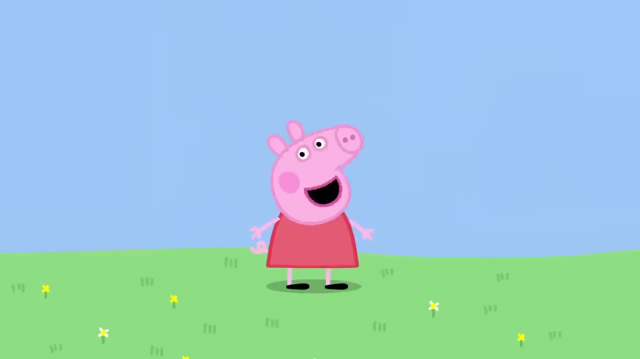 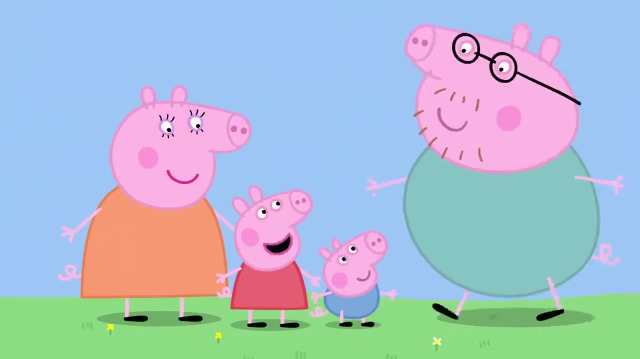 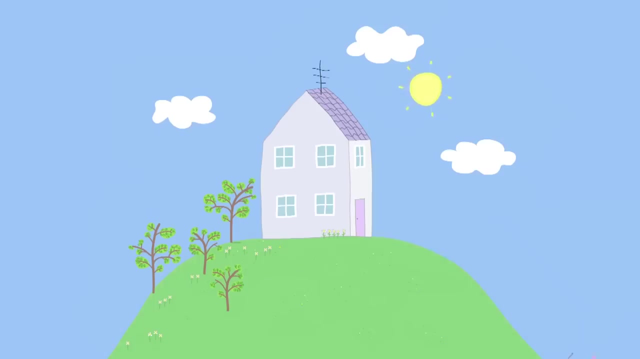 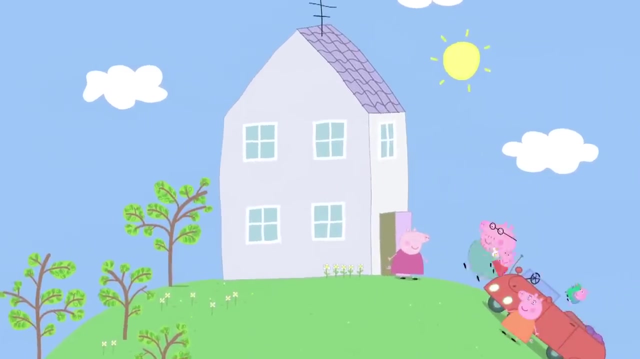 I'm Peppa Pig, This is my little brother George. This is Mummy Pig And this is Daddy Pig. Peppa Pig Gardening. Peppa and George are playing at Granny Pig and Grandpa Pig's house.